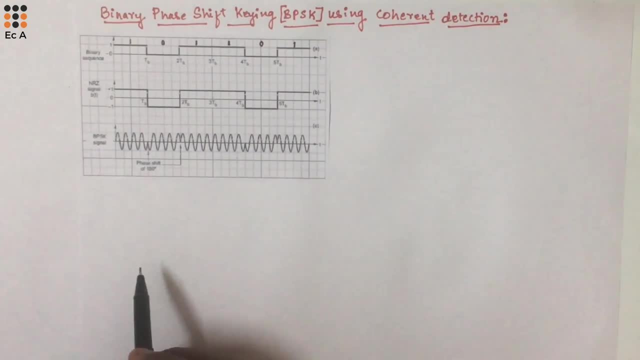 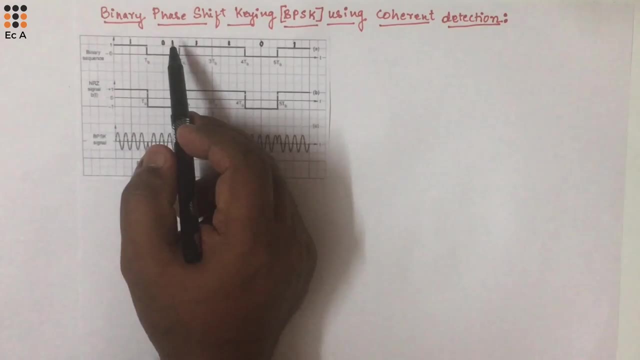 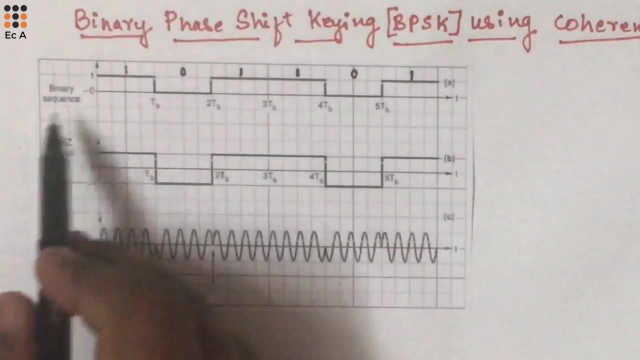 of the carrier at the transmitter. So here we will first understand the representation of BPSK sequence And then we will derive the mathematical expression for BPSK signal using coherent detection. This figure shows the representation of BPSK signal with respect to the binary sequence. 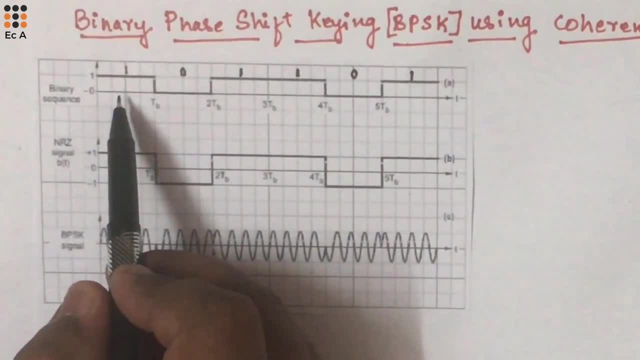 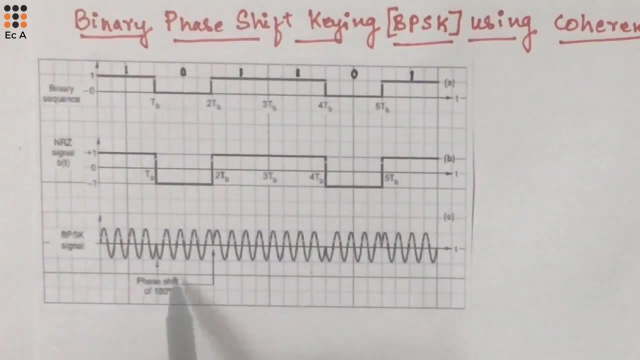 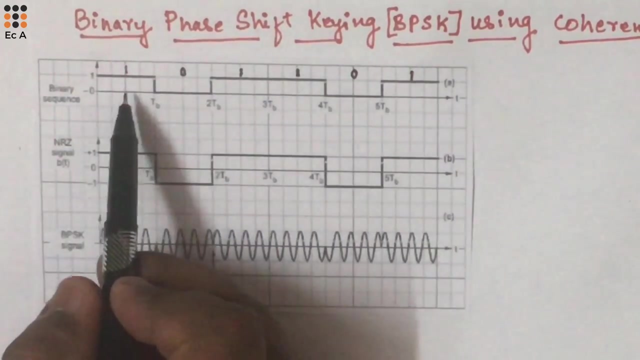 In phase shift keying, we know that when there is a transition from 1 to 0 or 0 to 1, there should be a phase shift of 180 degree. Let us take the binary sequence 101101.. As an example for this, the first step is to write the equivalent NRZ, which is non-return. 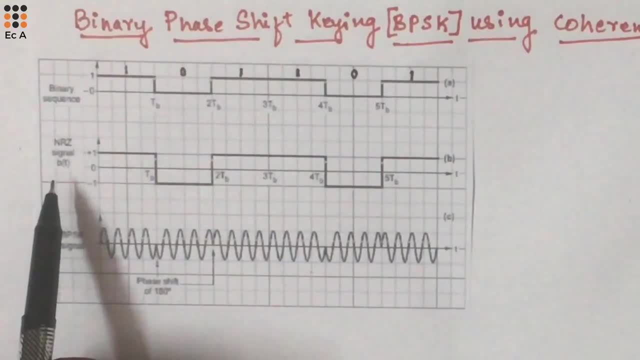 to 0 signal. In non-return to 0 signal, 1 will be represented with plus 1 and 0 will be represented by minus 1.. So for the sequence 101101, we will get NRZ at the signal as 1 minus 1, 1, 1 minus 1 rules. 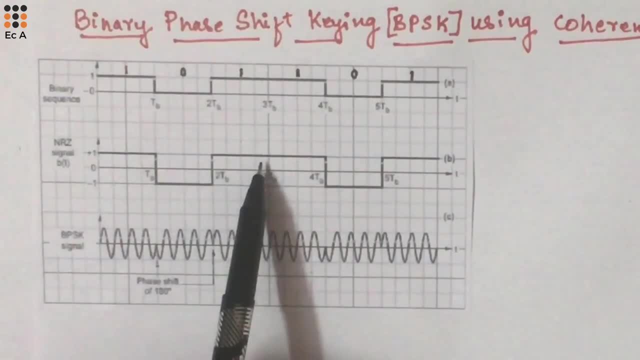 compress and turns on. As you can see by the middle of the phrase, nothing happens. here there is a tick normalization in the value of 1 and the negative sign. then the shape of two binary sequence will have a bonus function of 1 plus 1 and a negative sign of 2.. 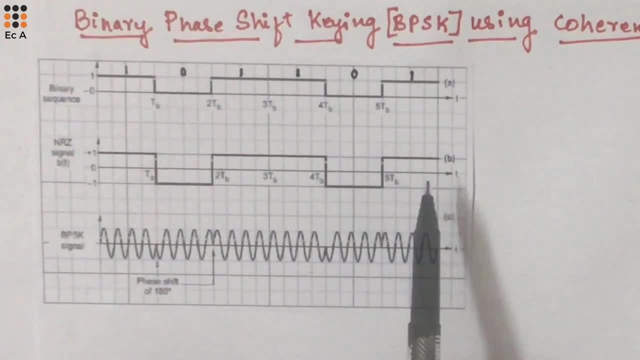 So we are in 5% wave state now, which means the momentum will be partly divided by 3-1 and 2, 1-1 numbers minus 1 and 1.. After obtaining the NRZ signal, this NRZ signal will be multiplied with the. 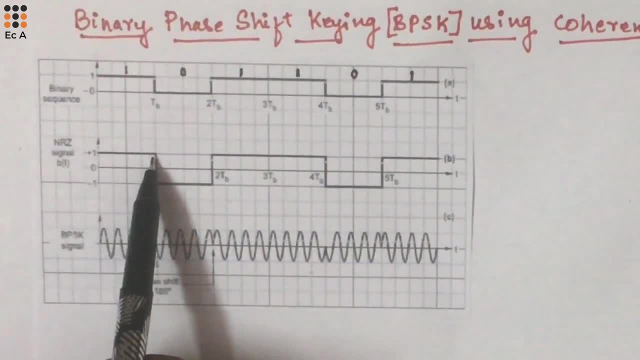 carrier signal. Now, if we multiply plus 1 with the carrier signal, we will get the carrier signal as it is. and if we multiply minus 1 with the carrier signal, at that case we will be having a phase shift of 180 degree. So 1 multiplied with the carrier signal, we will get the signal as it. 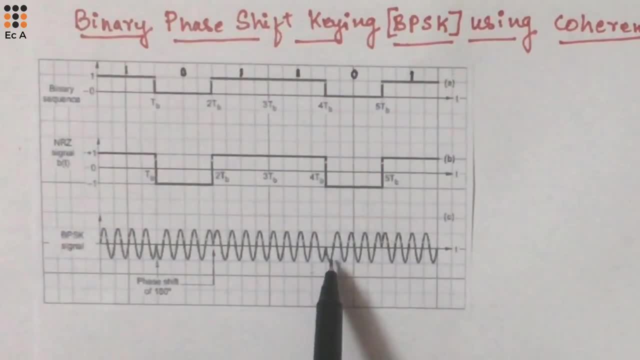 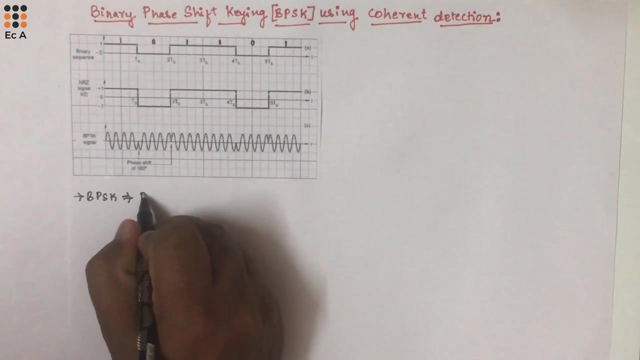 is and minus 1, multiplied with the carrier signal, we will get a phase shift of 180 degree. So this is how we will obtain the BPSK signal: using the binary sequence. In BPSK we use binary symbols, 0 and 1, and these binary sequence are used to modulate the phase of the carrier. Now let us 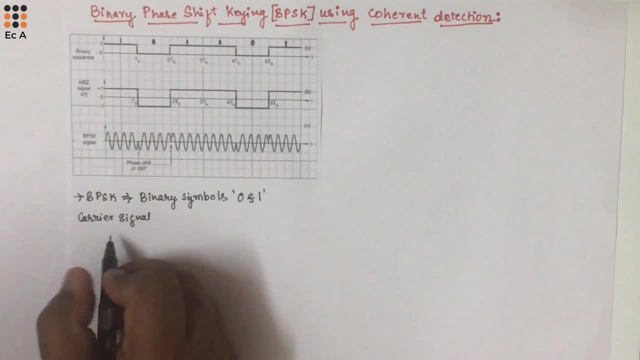 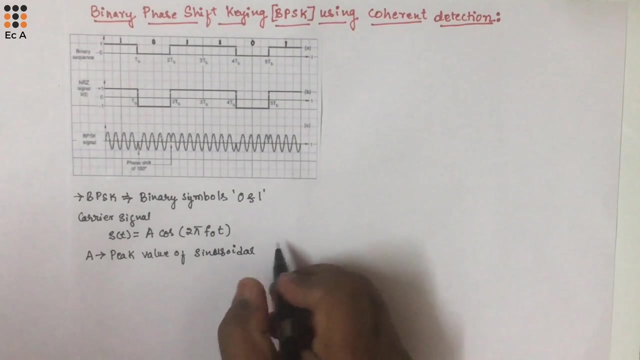 consider a carrier signal which is represented by the carrier signal. So let us consider a carrier signal which is represented as: S of t is equal to A cos 2, pi, f0, t. So this is the general representation of sinusoidal signal. Here A represents peak value of sinusoidal carrier. 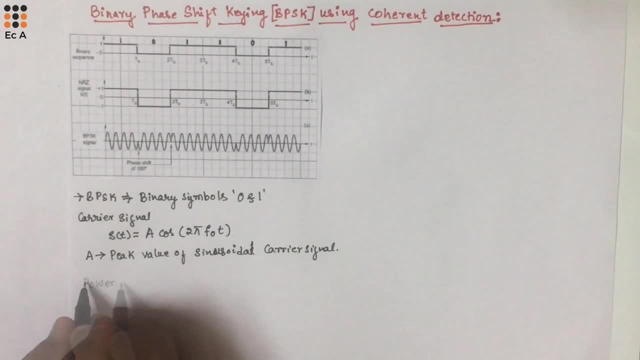 signal. Now the power dissipated by the signal can be written as: P is equal to 1 by 2 A square. So from this we can obtain: A is equal to square root of 2 P. Now we know when the symbol changes from 1 to 0 or 0 to 1, there will be a phase shift of. 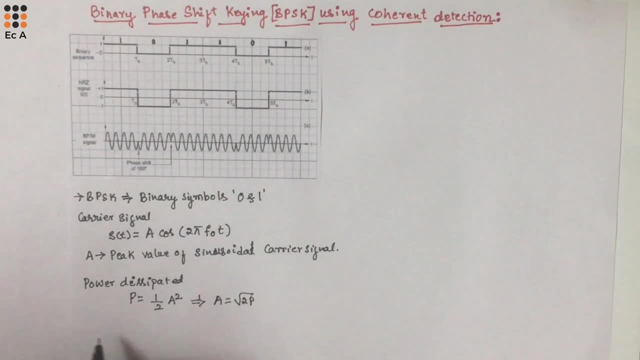 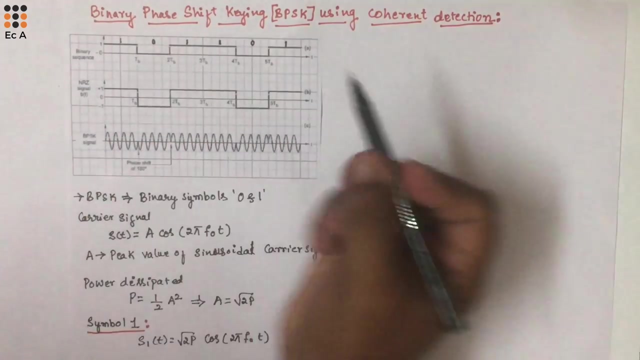 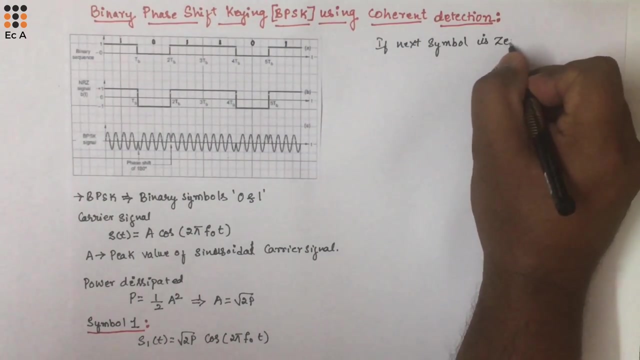 180 degree. Let us consider symbol 1.. We can represent the carrier signal as S1 of t is equal to. in place of A we can write root 2, P, cos 2, pi, f0, t After 1,. if the next symbol is 0, then for symbol 0, there will be a phase shift of 180 degree, which means we can write pi in terms of radians. 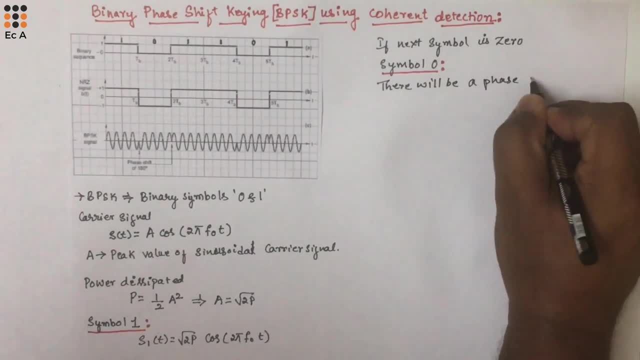 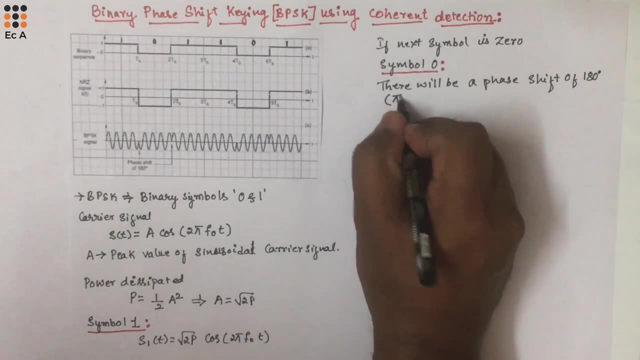 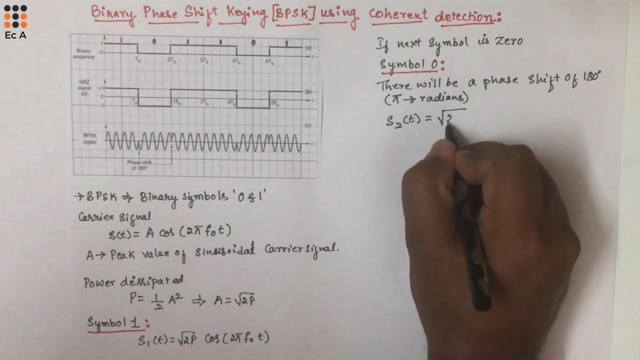 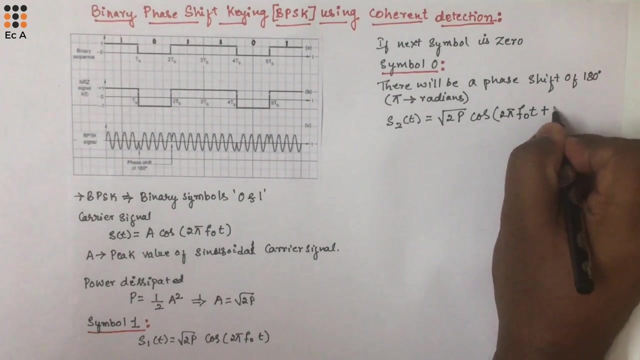 If the next symbol is 0, then for symbol 0, there will be a phase shift of 180 degree, which means we can write pi in terms of radians. So we can write the carrier, as S2 of t will be equal to square root of 2p, cos, 2pi, f0, t plus pi. 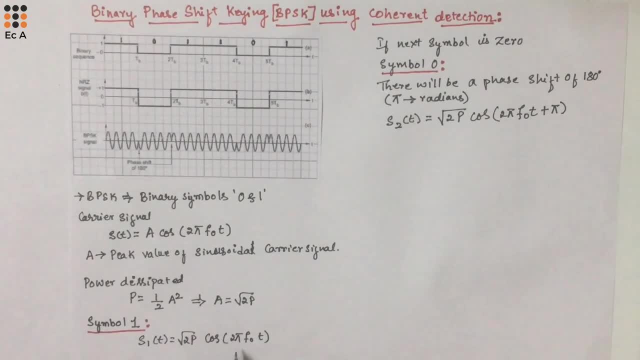 So the previous carrier signal was root 2p cos, 2pi, f0 t for symbol 1.. When the symbol changes to 0, there is a phase shift of 180 degree. So we will get the carrier signal as root: 2p cos, 2pi, f0 t plus pi.